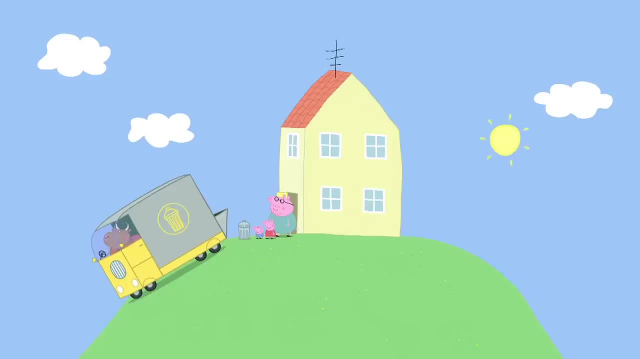 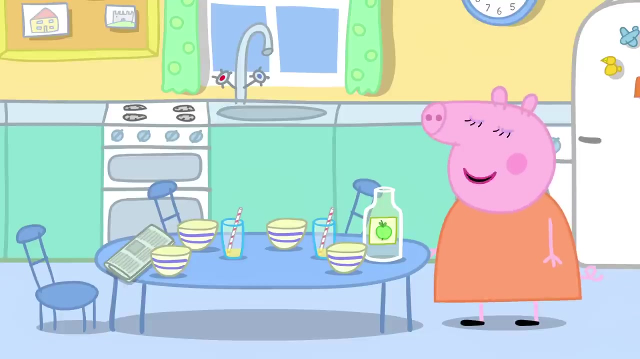 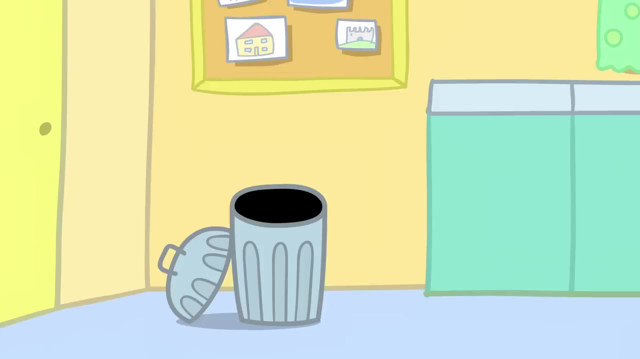 Bye, Bye. Mr Bull has emptied the rubbish bin for us. Good, Let's clear up the breakfast things. Can we help Mummy? Yes, you can. Let's throw this empty bottle in the bin, Peppa, stop. 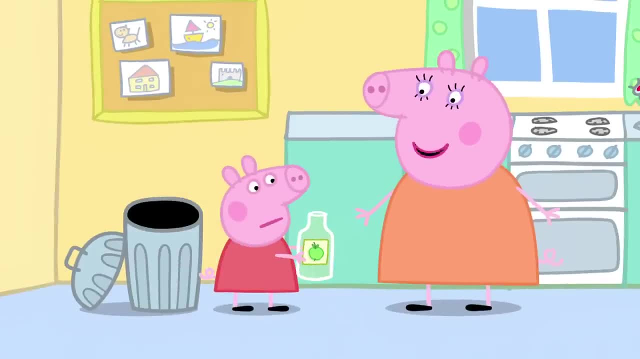 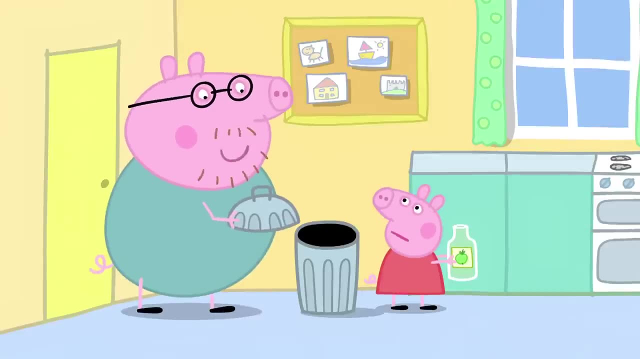 What? We don't put bottles in the rubbish bin. They can be recycled. What does that mean? All the things we can't use again, we put in the rubbish bin for Mr Bull, But all the things that can be used again. 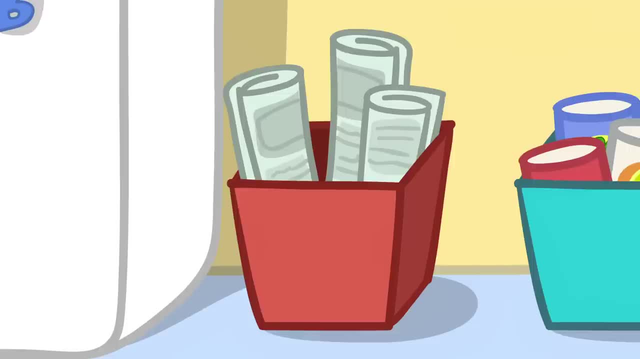 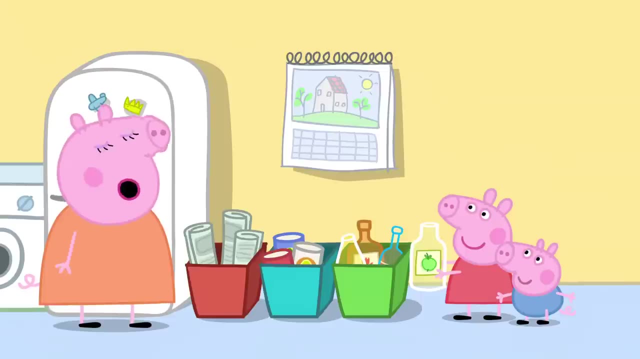 are put in these recycle boxes. The red one is for newspapers, The blue one is for tin cans And the green one is for bottles. Peppa, you have a bottle, So which box does it go in? Um, the green one. 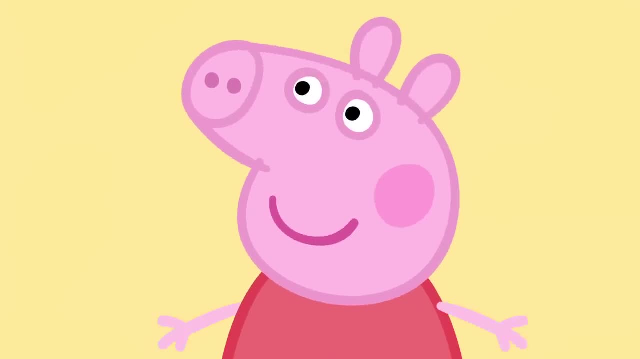 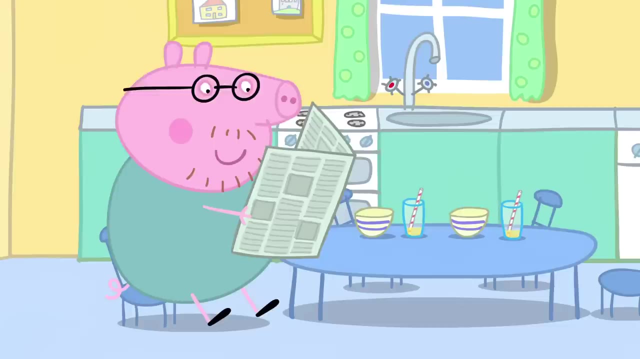 Yes, This is fun. Now it's George's turn. Can you find a newspaper for the red box? Peppa and George laugh. George wants a newspaper. George wants a newspaper. George wants to recycle Daddy Pig's newspaper. Ho ho. 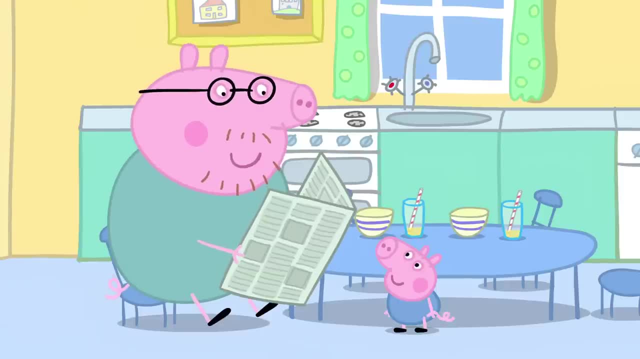 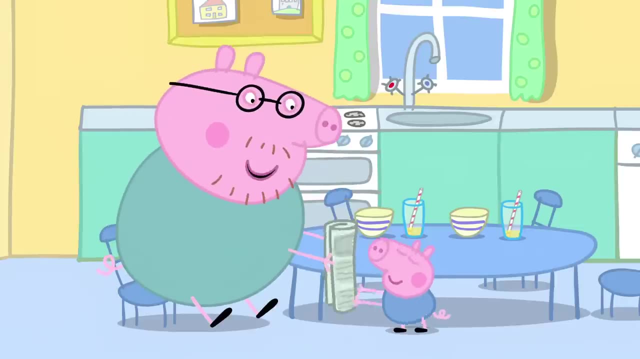 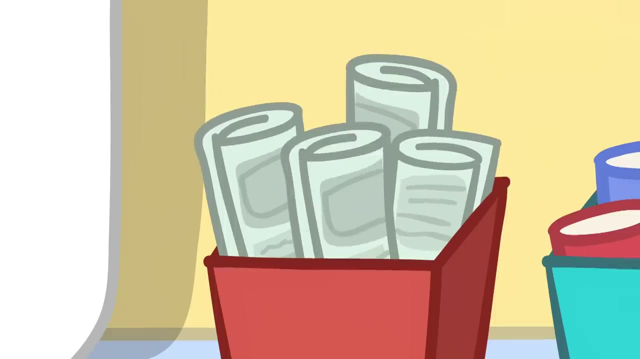 I haven't finished with my newspaper just yet, George. You can have it in a minute. Oh, all right, Here you are, George. Newspapers go in the red box. George, Now that we have collected enough things, we can go to the recycle centre. 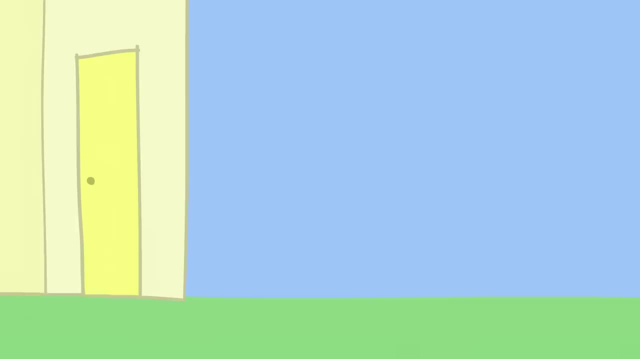 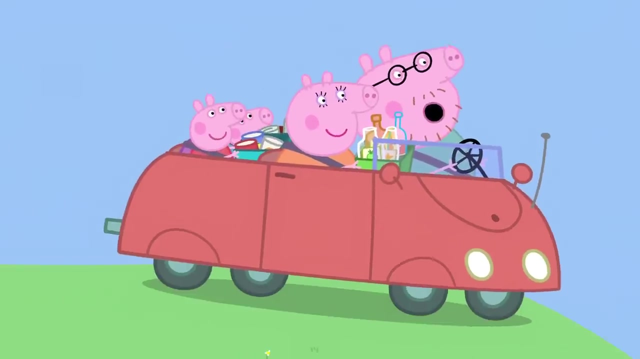 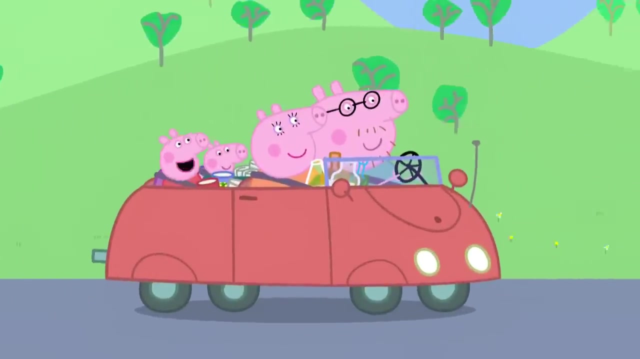 Hooray, Let's go. Mummy Pig has the bottles, Peppa has the tin cans And George has the newspapers. Is everybody ready? Yes, Daddy Pig. Then let's go. Recycle, recycle, We're going to recycle. 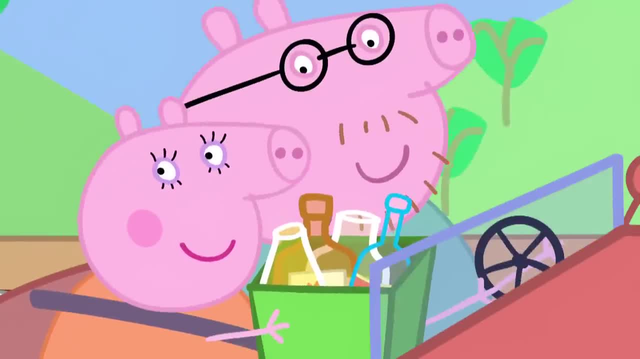 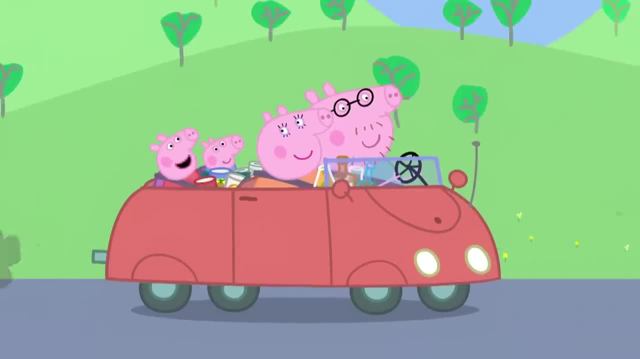 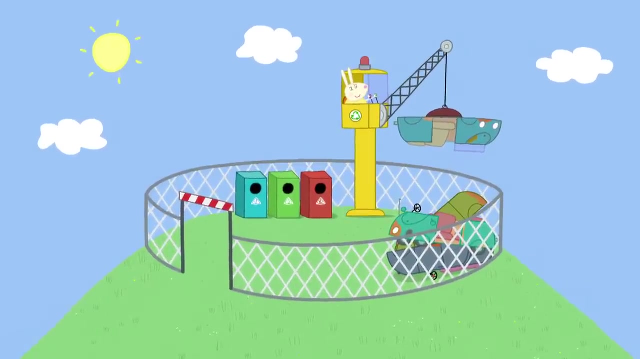 Tin cans, Portal Newspapers. Yes, Recycle, recycle, We're going to recycle. This is Miss Rabbit's recycle centre. We're here, Hooray, Hello there. Hello, Miss Rabbit, Have you come to do some recycling? 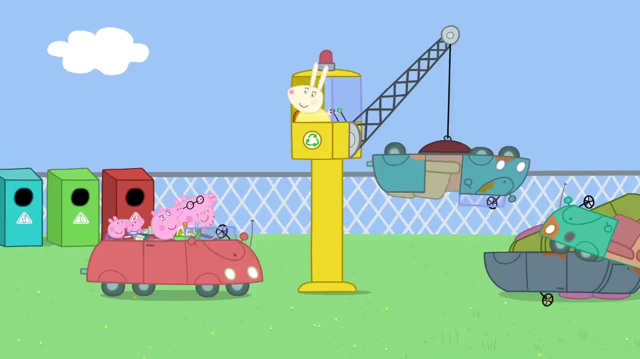 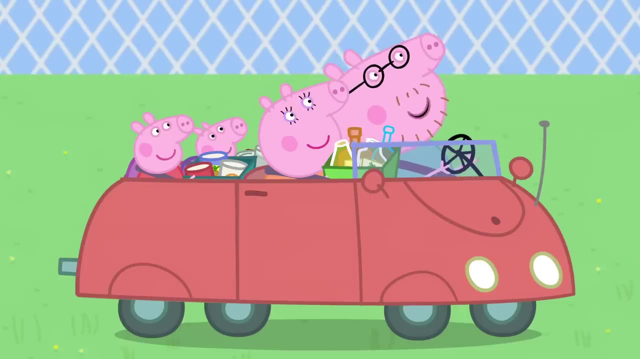 Yes, we have Jolly good Carry on. What's Miss Rabbit doing? She's recycling. All right, Let's go. Let's go. Hooray, Hooray, Hooray, Hooray, Hooray.